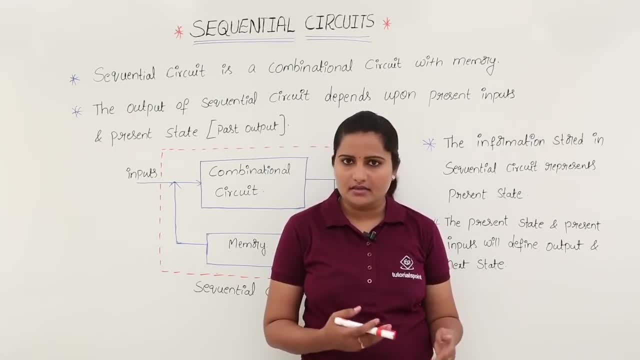 So previously we taken the introduction and some applications of combinational circuits. So here combinational circuit output is dependent upon only present input, it is not having any memory. but sequential circuit is always a combinational circuit with memory. That is the difference between combinational and sequential. Whatever. 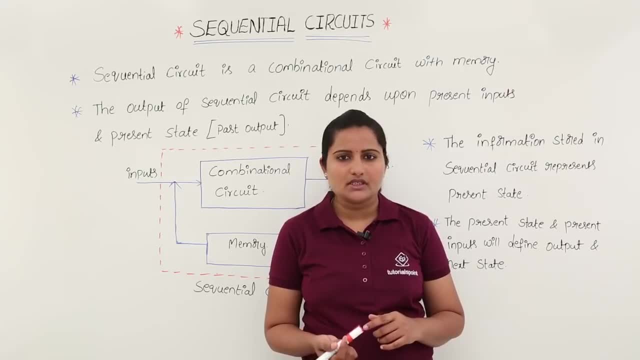 things, that is, we are going to do with combinational, we can do with sequential, and the extra things we can do is we can maintain memory. here that means combinational circuit with memory is called a sequential. So here in this, the output of sequential 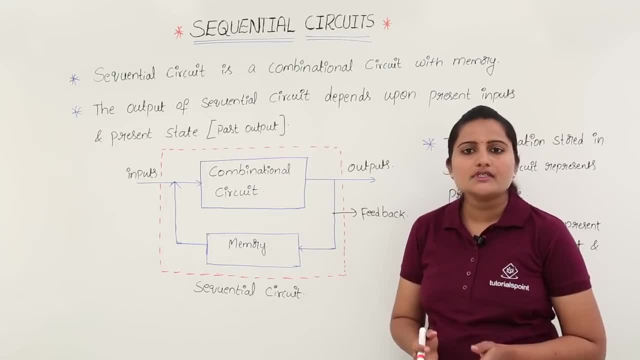 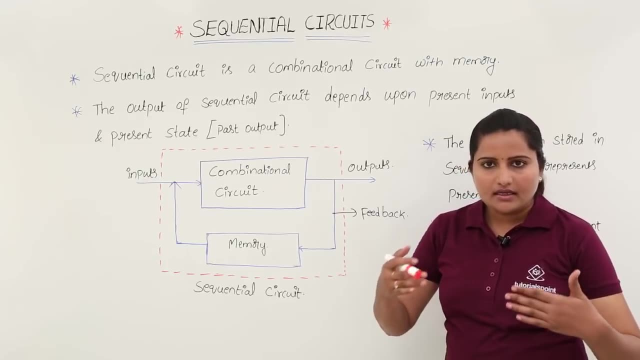 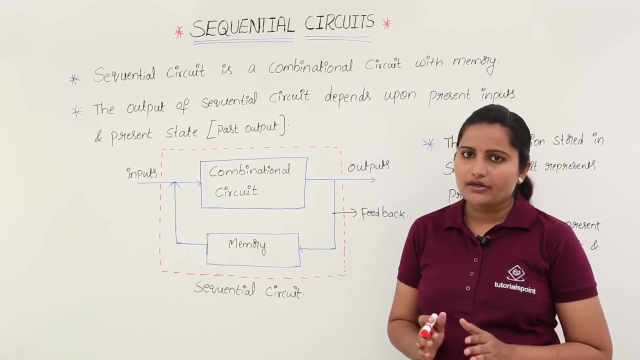 circuit is always depends upon the present input and present state. Present state of machine is dependent upon past inputs. only We are in this state means that is because of past inputs or past outputs. So our sequential circuit output is dependent upon present inputs and present state. that present state is nothing. 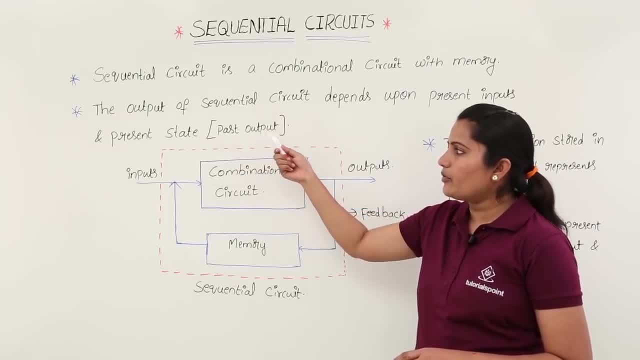 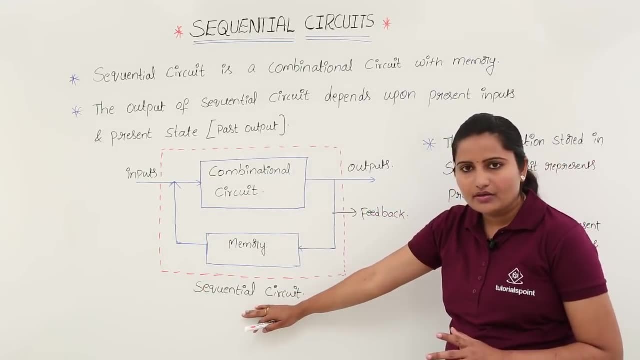 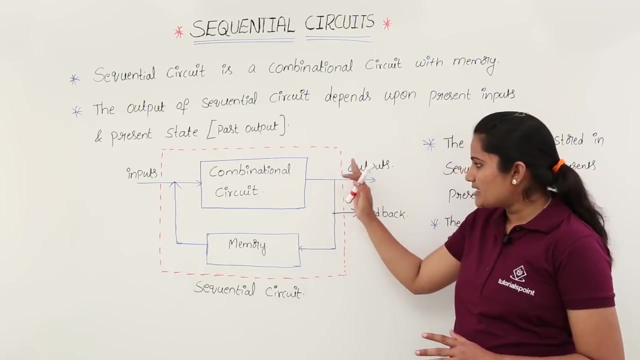 but that is that implies that that is dependent upon past outputs or past inputs. So here this is the block diagram of your sequential circuit. So here you can observe this is a combinational circuit with memory as your feedback, Whatever present state is there. 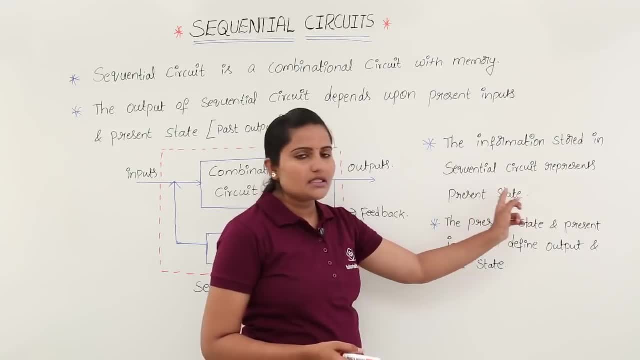 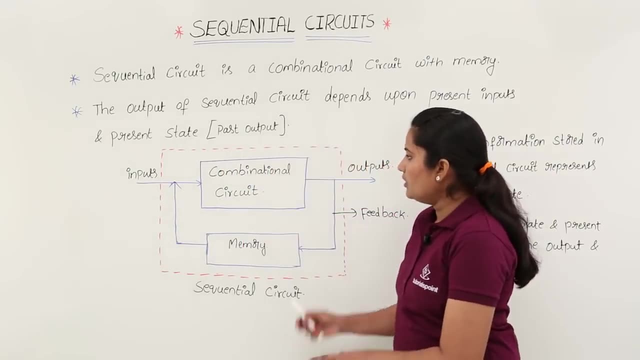 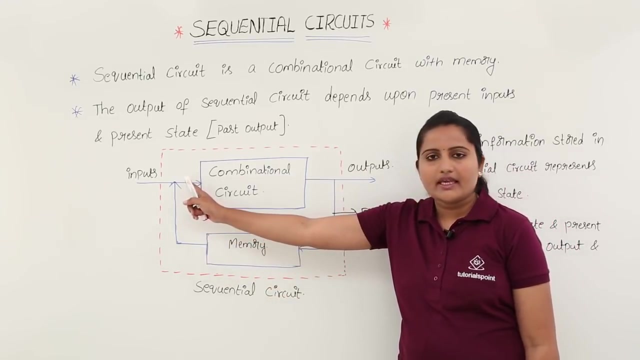 present state is nothing but the information stored in sequential circuit at particular point of time is called as its present state. For example, now the combinational circuit output that we are taking as present state, that present state we are giving as present input. with our new inputs that means present inputs. we are getting our output If output. 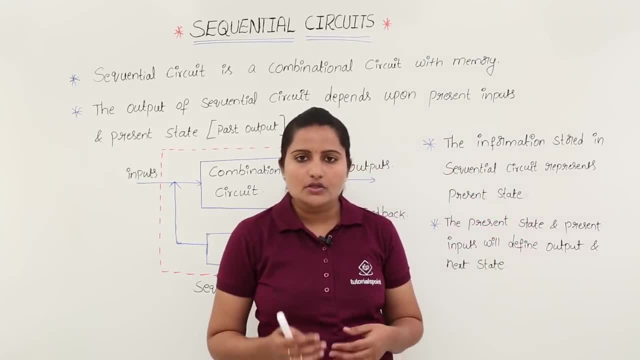 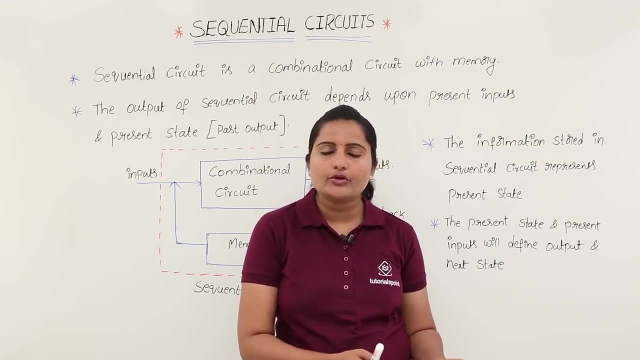 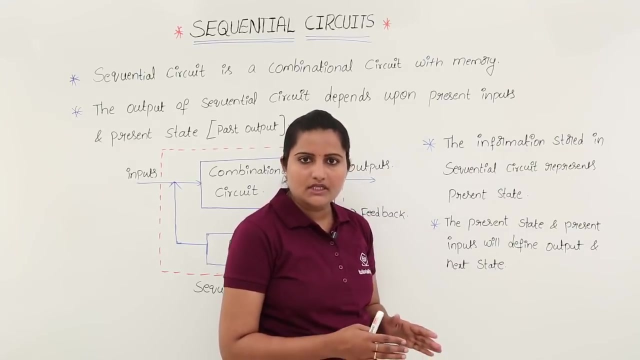 is defined next state also. we can define So in the circuits of sequential circuit. so I will show you how we are going to take the main output and its next state. So by defining present state, the actual state of sequential circuit at particular instant of 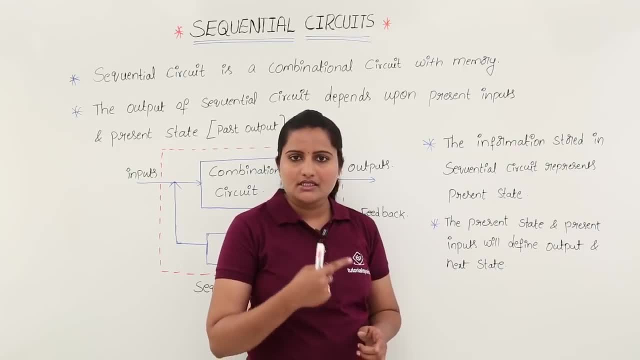 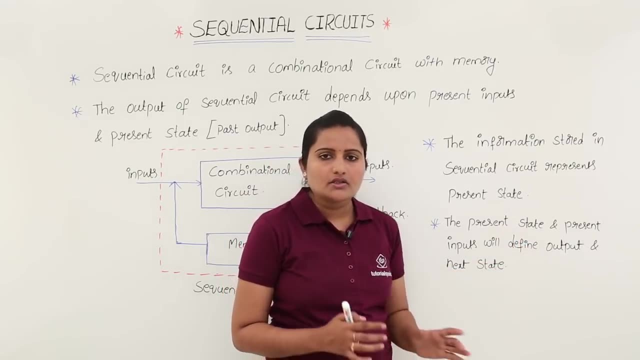 time is called as present state. So by taking the reference state we are getting our output. So by taking the reference of that present state with present inputs, we are going to get output and its next state. So this is about sequential circuit. So these are classified into two types, that is. asynchronous and synchronous. As the name indicates, synchronous sequential circuits runs with same clock pulse or similar clock pulse. Asynchronous sequential circuits runs with different clock pulse. that means whatever sequential element. So those elements are there. those elements are not going to use same clock pulse in asynchronous.